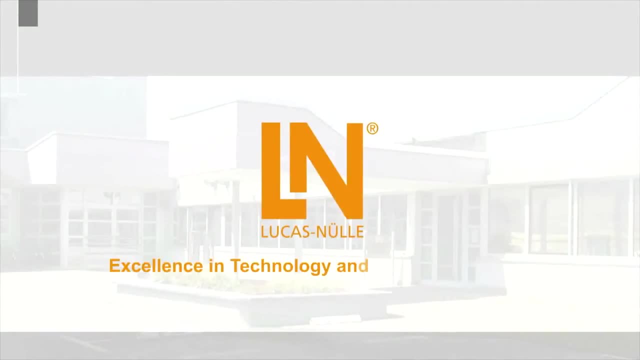 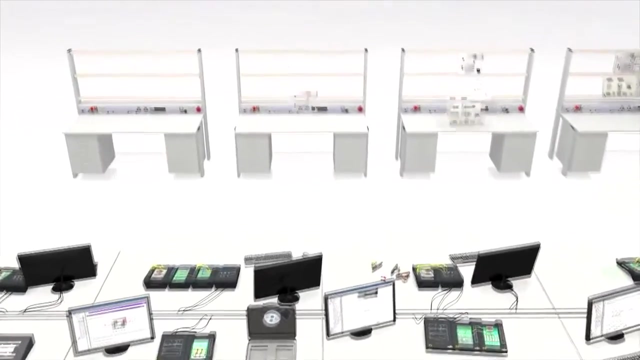 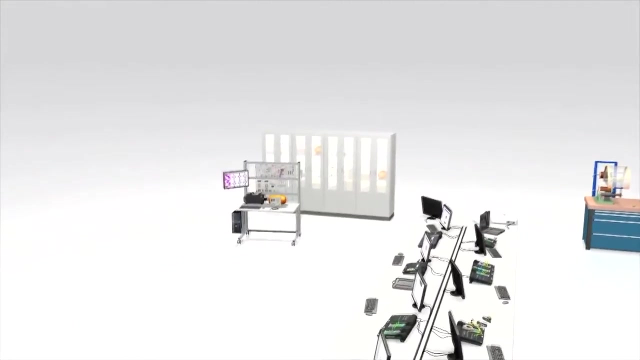 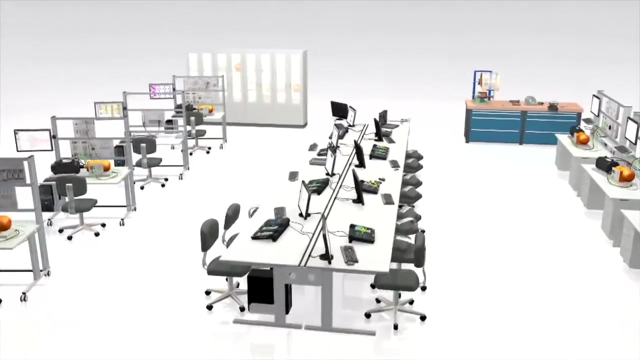 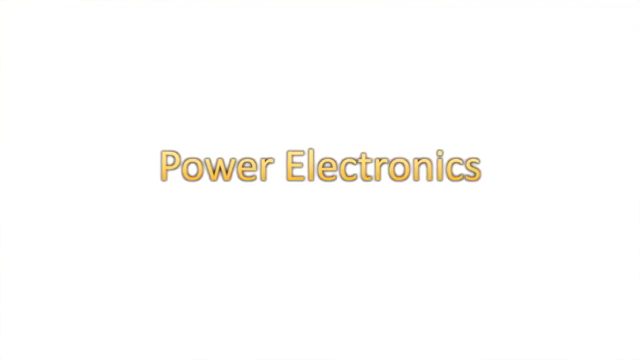 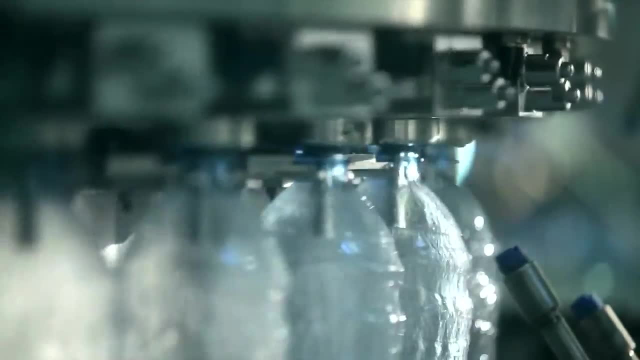 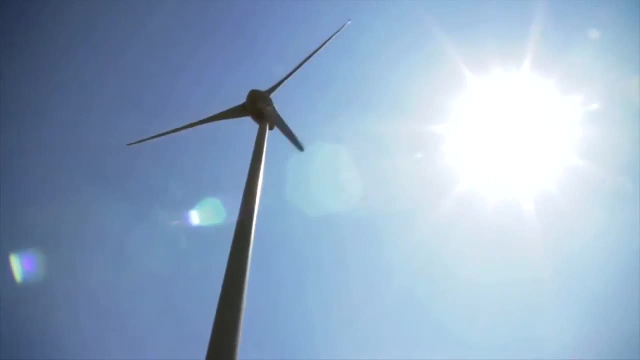 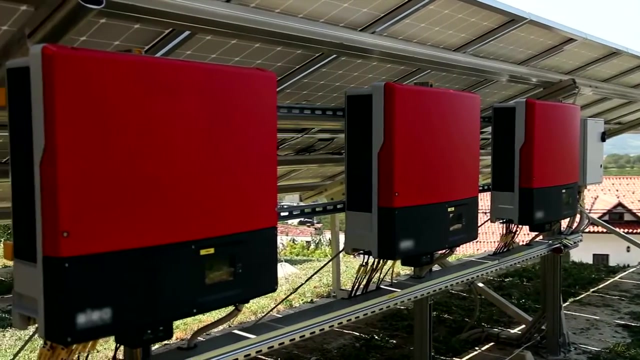 Everyday life without power electronics is no longer imaginable, At home or in the factory. Whether it be drive technology, Whether it be drive technology, renewable energies, power electronics plays a crucial role. This raises the bar in terms of what electrical engineers, technicians and engineers generally need to know, Because 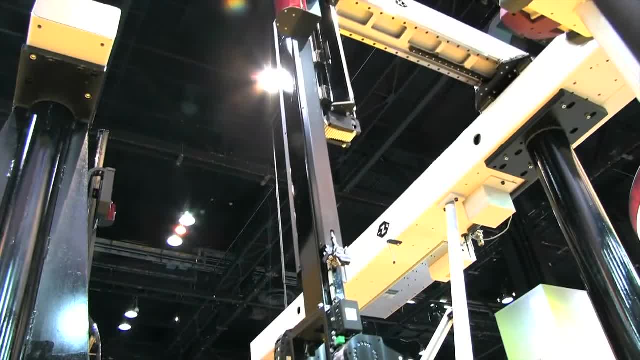 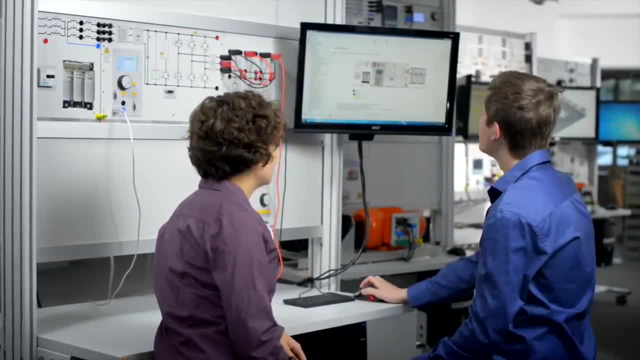 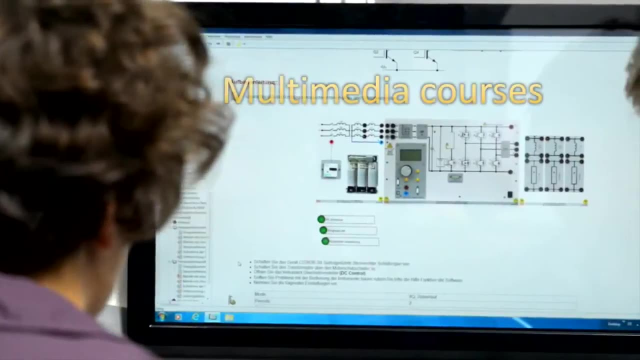 wherever and whenever power electronics is involved, highly qualified technical skills are in demand. The power electronics course from Lukas Nüller is ideal for vocational training. The multimedia course conveys basic and advanced know-how that is both graphically appealing, technically up-to-date and includes lots of experiments. This training system also lets 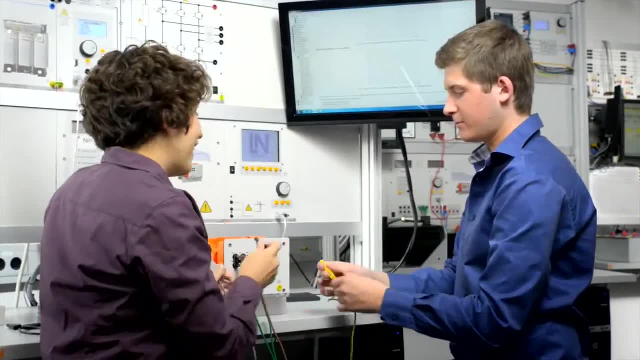 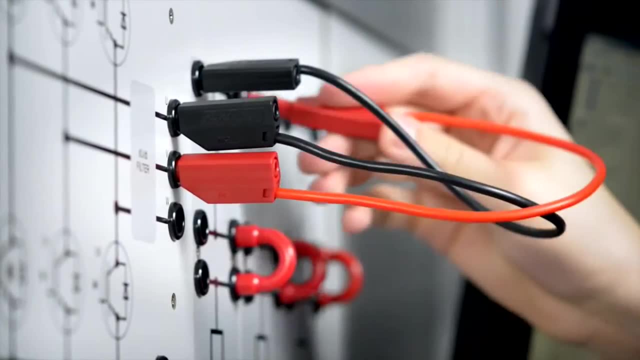 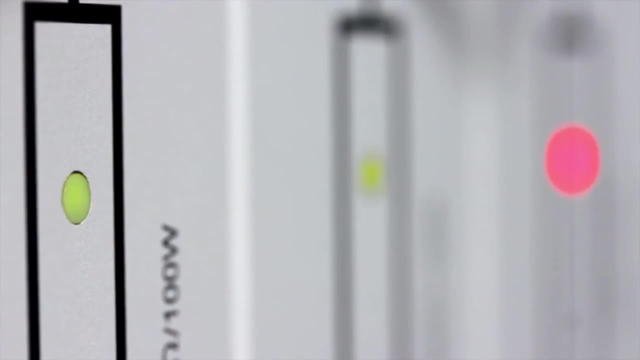 you put the theoretical knowledge that you have learned to practical use. Lots of different experiments make power electronics understandable. To achieve this, the training equipment has been modified especially for educational purposes, which facilitates rapid learning, success and motivation. Adding supplementary modules is child's play and serves to deepen what has 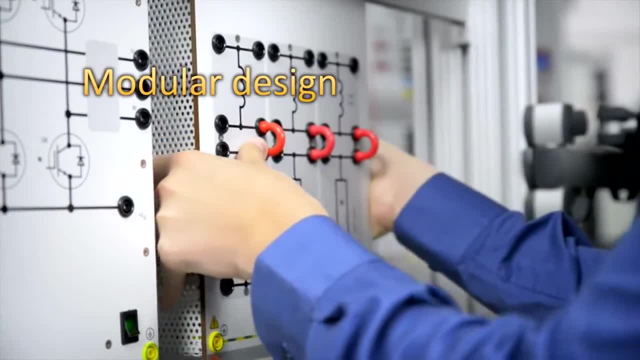 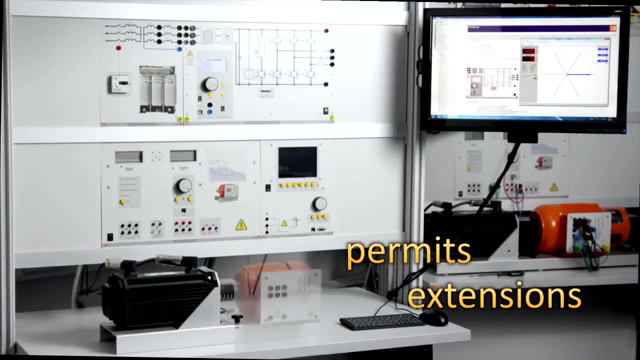 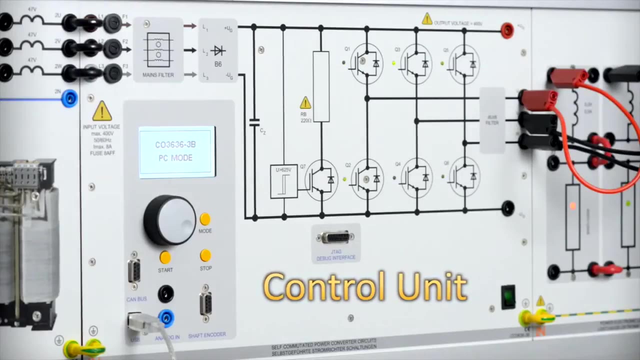 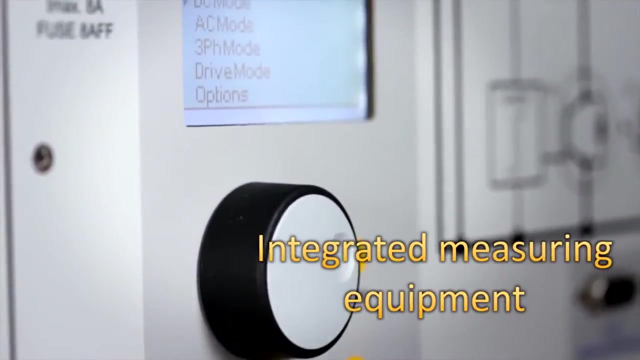 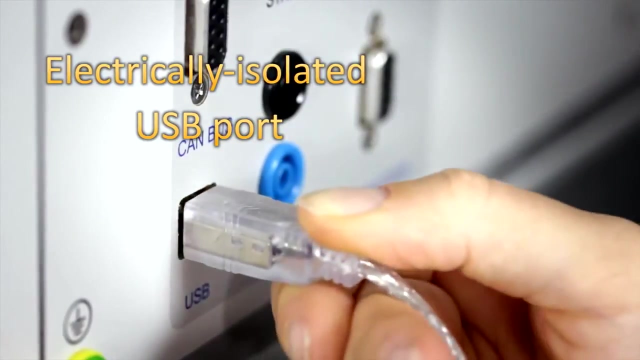 been learned. Thanks to this modular design, the system can incorporate a variety of experiments ranging from beginners to advanced levels. One essential element is the control unit. It contains the power electronics and the instrumentation. An electrically isolated USB board ensures interference-free data transmission to the PC. The software integrated into the multimedia course. 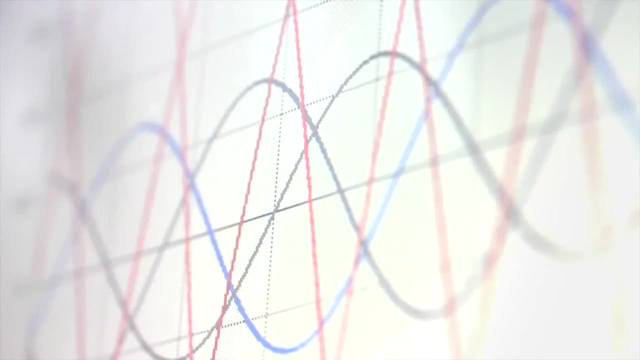 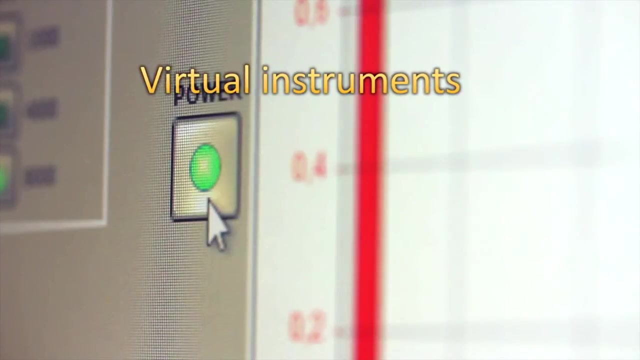 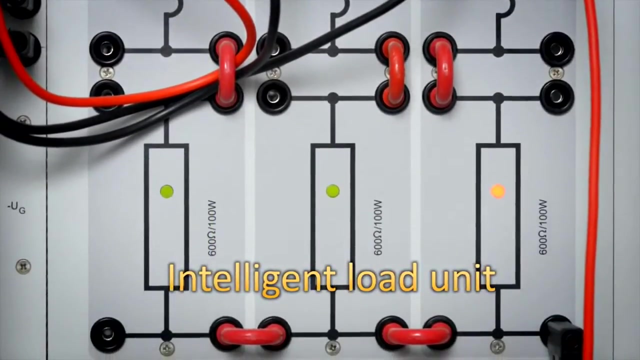 allows you to evaluate the experiment results. This software includes numerous integrated measuring instruments, thus rendering the purchase of real meters superfluous. With the intelligent load unit, a host of different consumers are simulated for the experiments. The visual display is an aid to both understanding and learning. 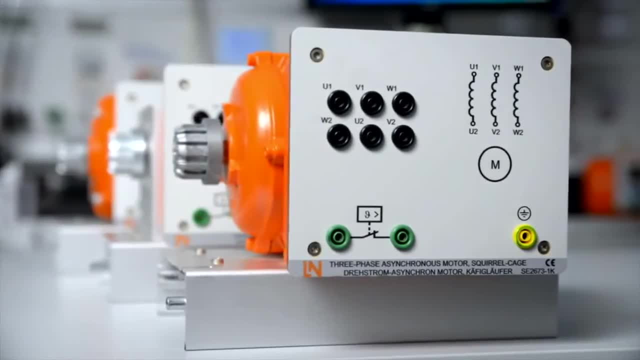 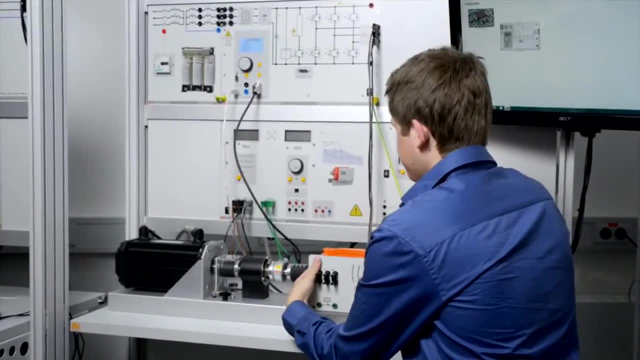 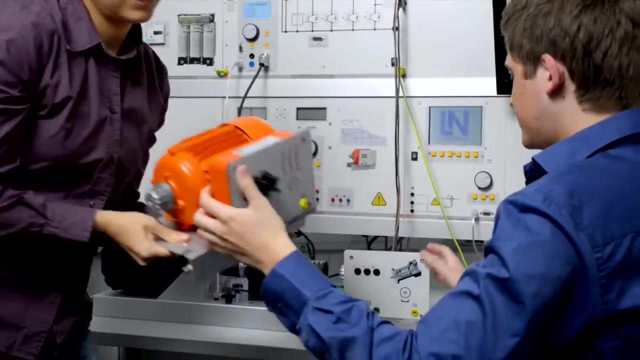 The system offers various motors with power levels of 300 watts or 1 kilowatt for the assembly of drive units. These motors are then investigated and optimized by the students using the servo machine test stand. The experiments are totally safe for the students. 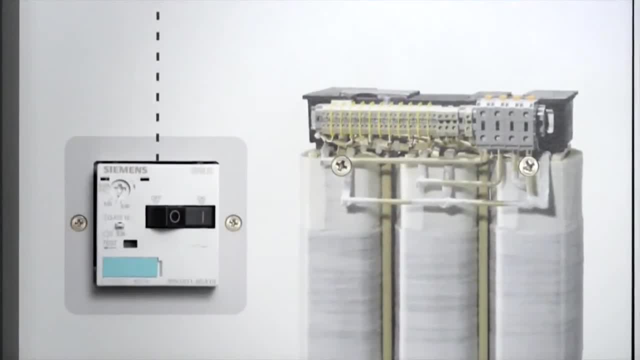 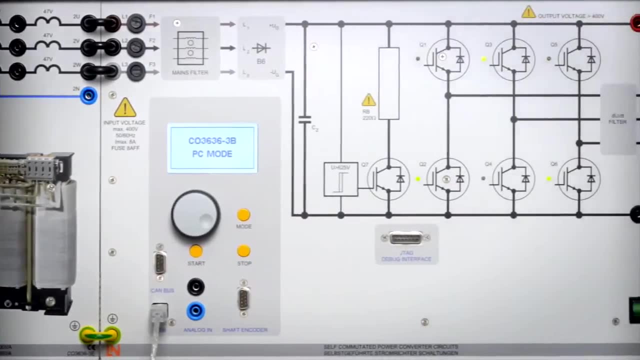 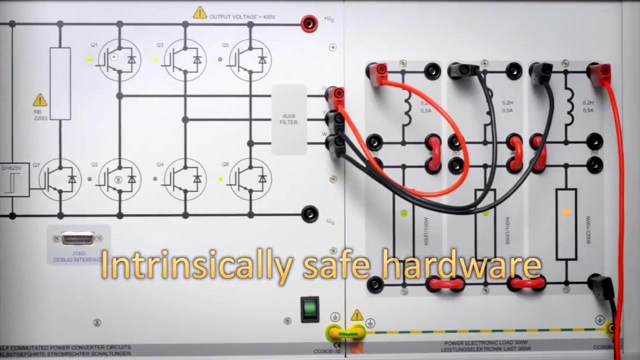 The isolating transformer decouples the system from the mains. The control and load unit switches off automatically, for example in the event of excessive amperage, and thus protects not only the student but also the device itself. Students can create and run sophisticated programs using the MATLAB and Simulink programming languages. 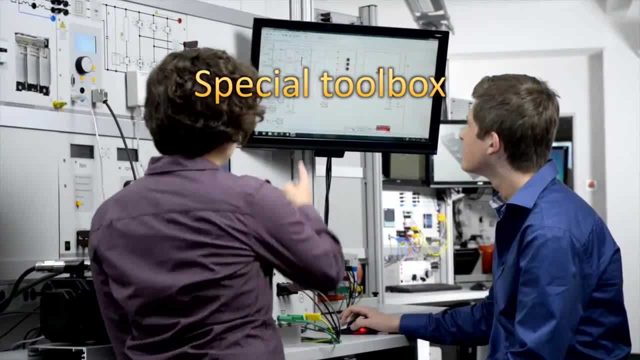 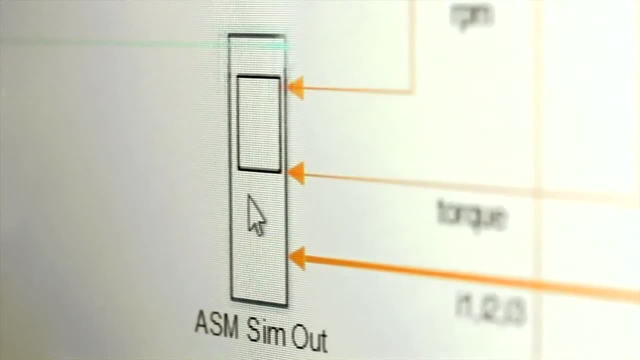 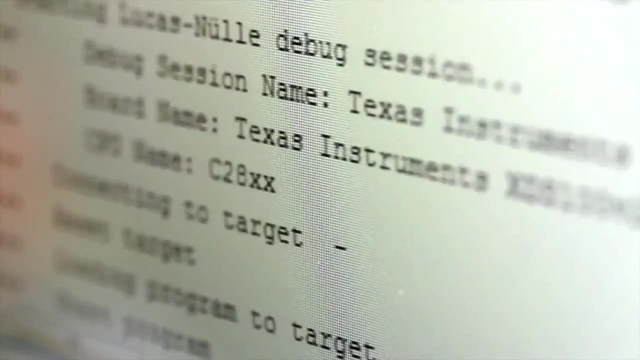 Getting started is quick and easy thanks to the specially designed LucasNuller Toolbox. This makes pre-installed templates for the hardware settings available from the start, so that students can immediately begin programming. After simulation on the computer, students can upload the programs to the hardware. 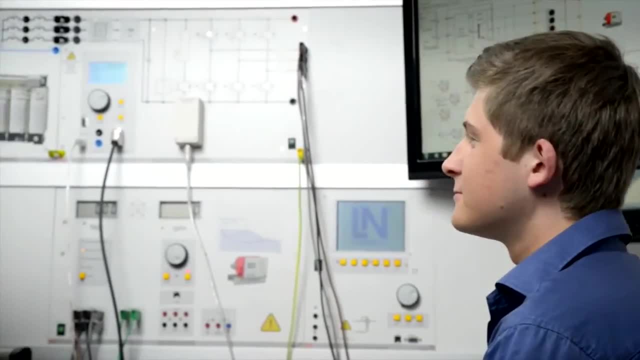 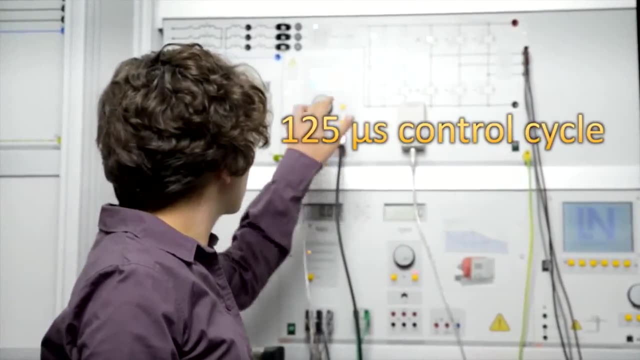 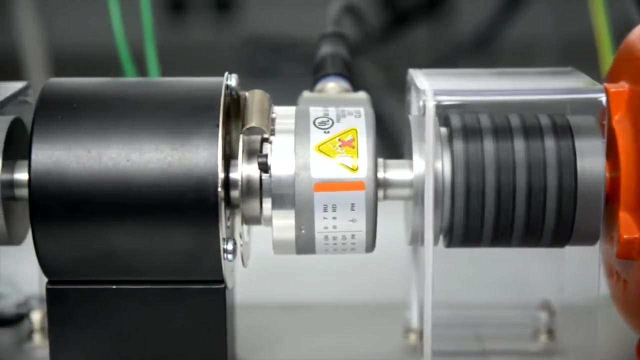 This way, they can test various control loops using a real converter with a motor and a load. The control unit delivers rapid control cycles of 125 microseconds. That's why the system can respond to different measurement values without any delay, even when dealing with complex algorithms. 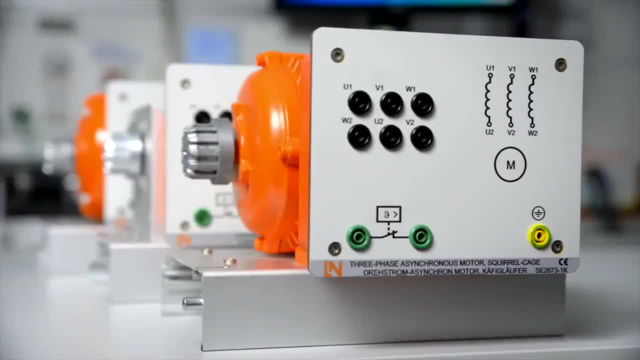 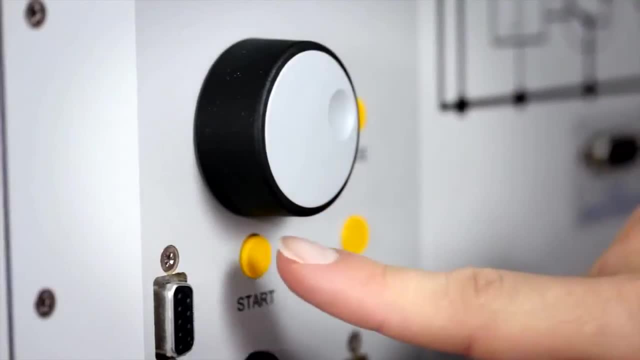 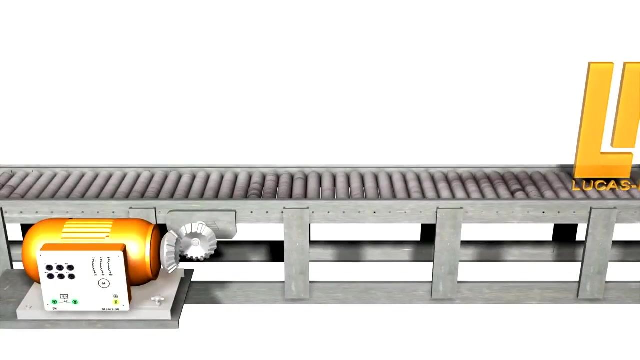 Fine-tune the equipment to your training needs for beginners or advanced. Use the Power Electronics training equipment from Lucas Nülle to learn, experiment and understand. Learn more at LucasNüllecom.